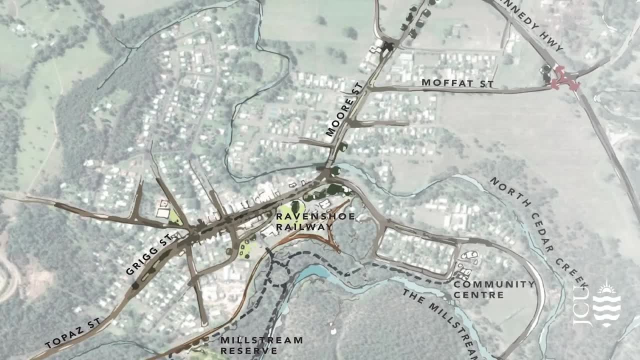 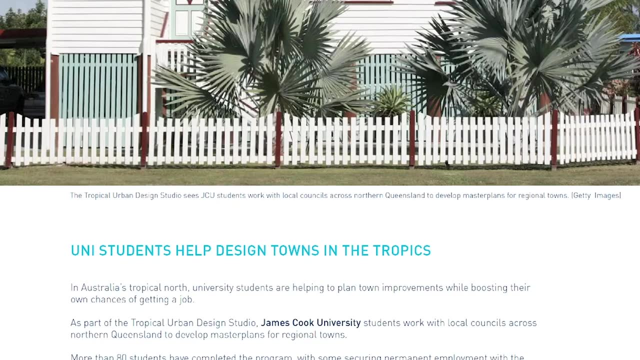 this in Ingham and in Innisfail and in Ravenshoe. We were recently listed in the University's Australia Guide for Work-Integrated Learning and it's fantastic to be acknowledged that our students are getting Australian best practice in doing design work with these communities. 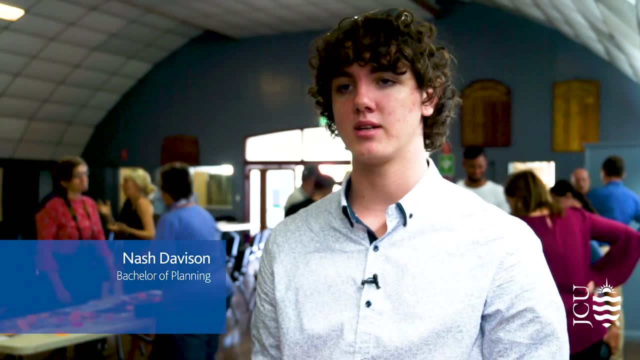 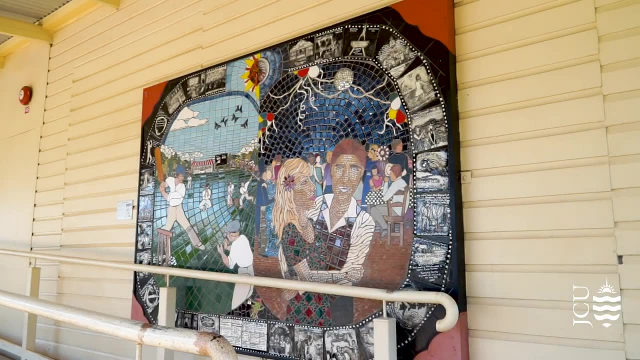 We're at the Melanda Showgrounds and currently we're working on the Melanda Master Plan. My group is doing the heritage of the town, which is important because this is a very old Australian town, Instead of sitting in the classroom and just reading off slides. 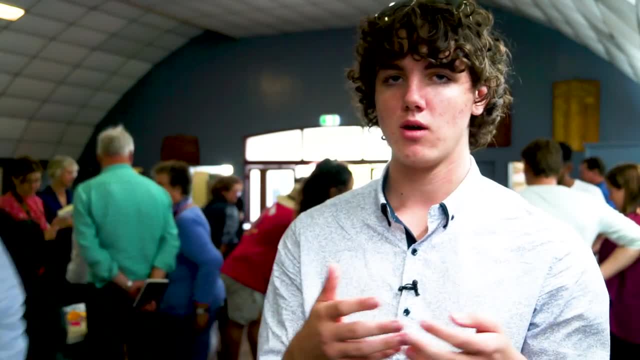 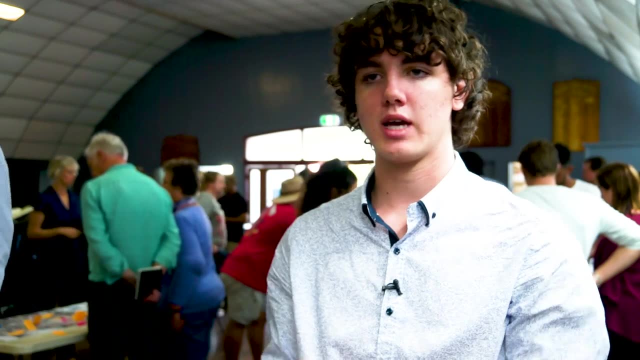 and board. I actually get to come out here and talk to people and understand what they want from a planner and understanding what I need to do if I go out and get this job, Especially with heritage- because I appreciate history, Coming out and talking to the original. 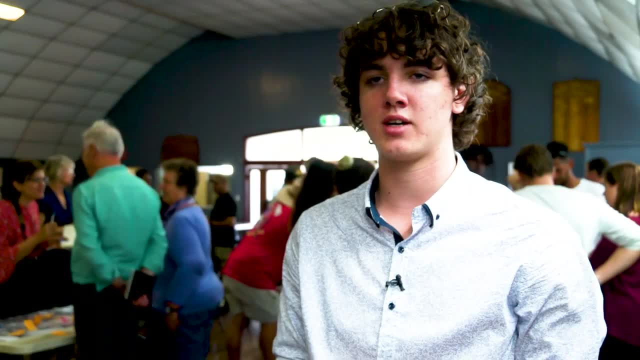 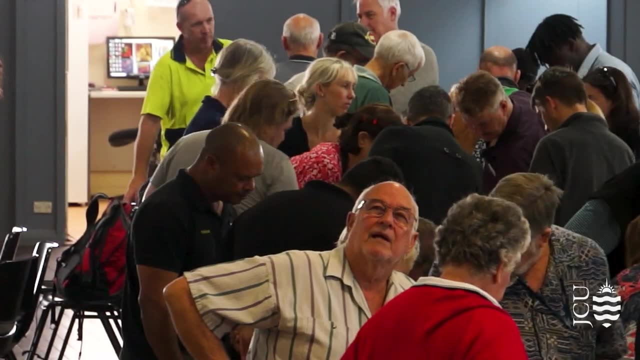 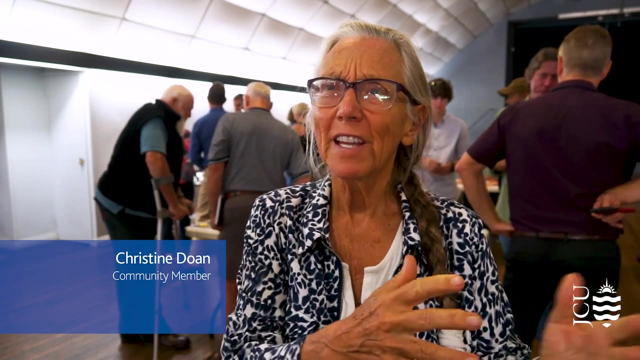 custodians, people who have lived in this town their entire lifetimes- and learning what makes this town, rather than what it looks like on Google Maps. What I really love is that we have some older professionals with experience and we have this whole group of young people who have new ideas, new consciousness. So they've got. 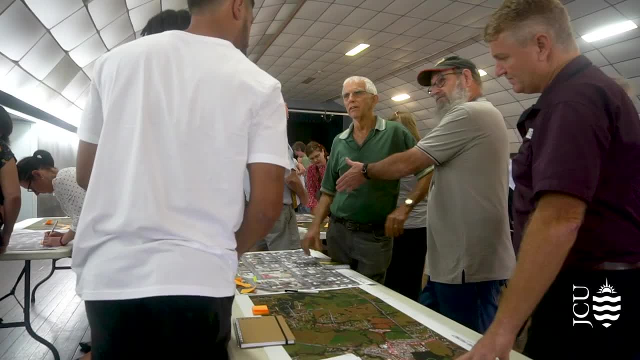 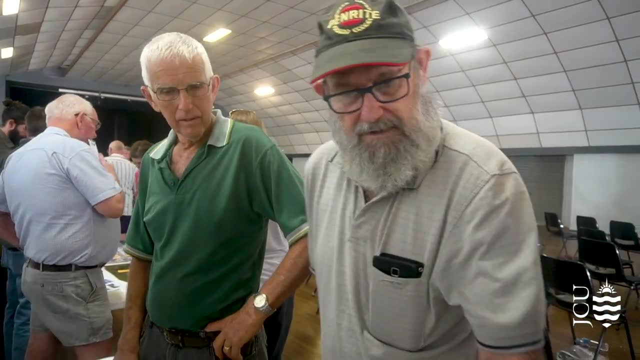 skill sets and mindsets that are different to a 70-year-old. I love it that JCU and the community are working together. People will be feeling that they are empowered to improve their community. I hope it's making other people feel as good as I feel about it. 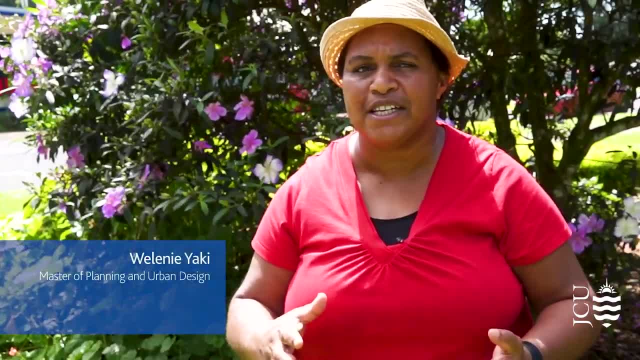 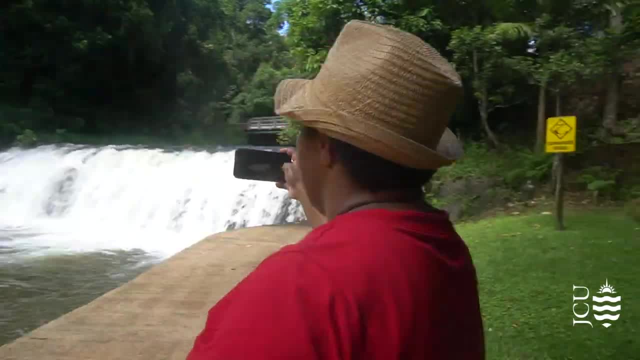 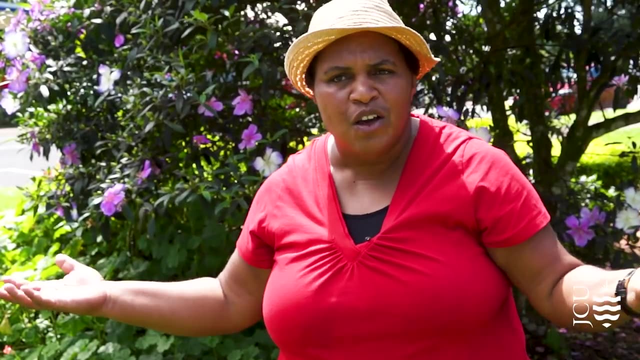 I'm doing research on young people. clearly It's really important for young people to, and kids especially. what are their needs? how can we incorporate them into the design process? Lisa and I came here on Tuesday and we interviewed the high school students and then they talk about like we don't want to stay here and like 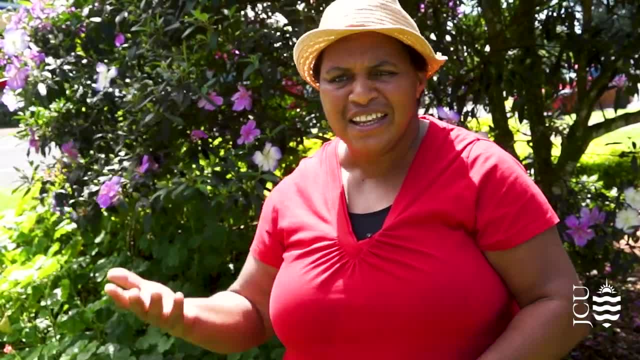 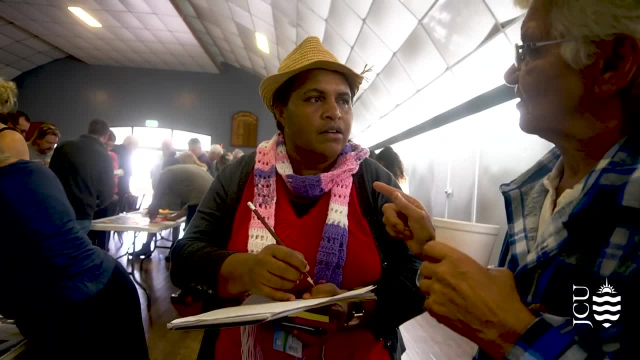 I asked them why you you don't want to stay here. and then you know those are the reasons that they gave will make our planning better for the future. yeah, I'm coming here to get my qualification, but at the same time I'm contributing to the 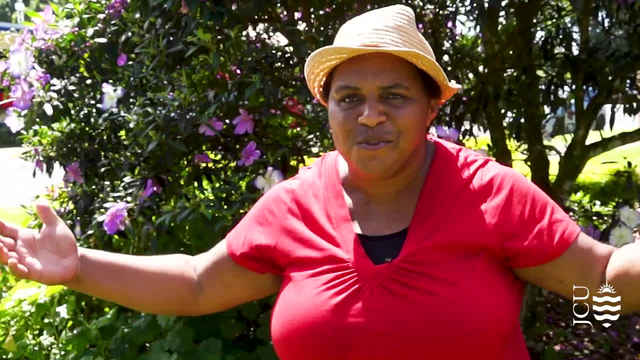 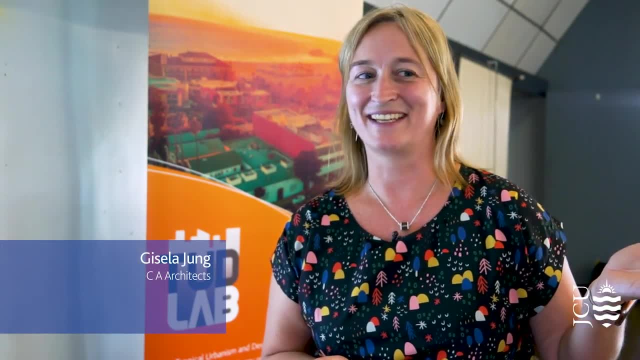 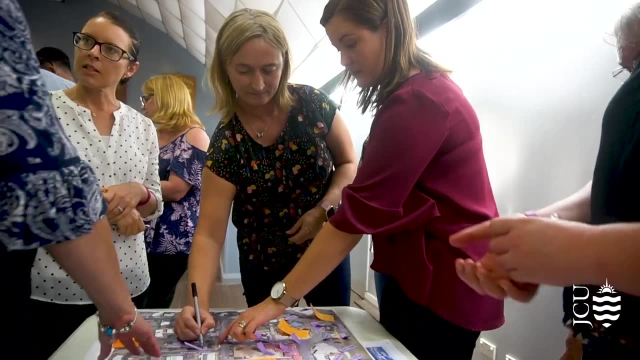 economy and the development of Australia, which I am super proud of it. yeah, It's an amazing community. they have been really active today, so we've had great feedback. this is only session one. Every table that I've joined had an amazing amount of ideas and I can already see the master plan forming. it's really exciting.